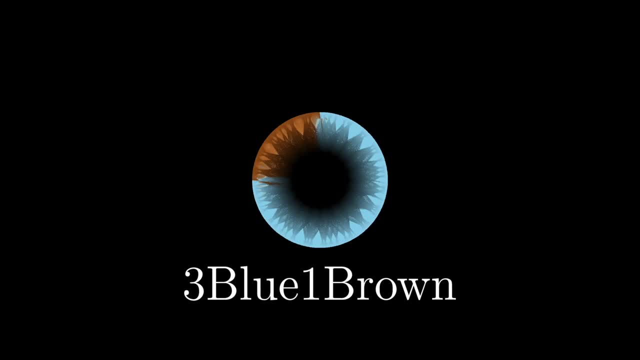 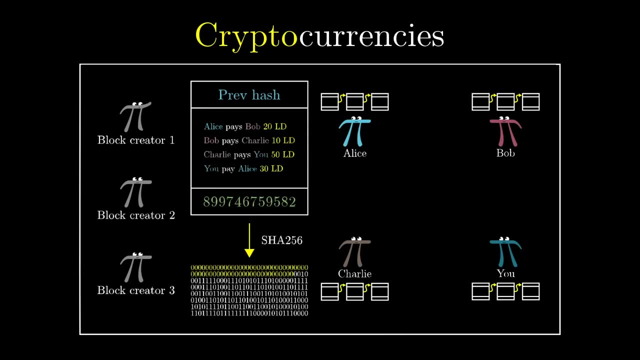 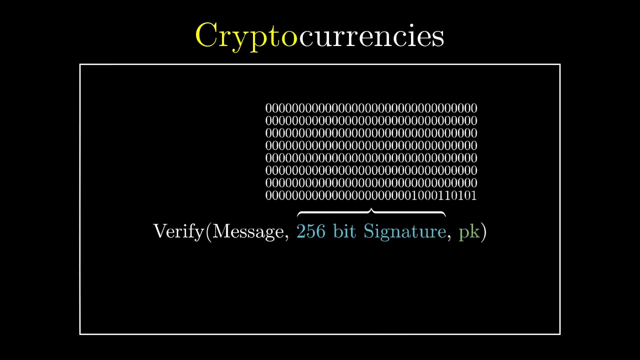 In the main video on cryptocurrencies, I made two references to situations where, in order to break a given piece of security, you would have to guess a specific string of 256 bits. One of these was in the context of digital signatures and the other in the context of 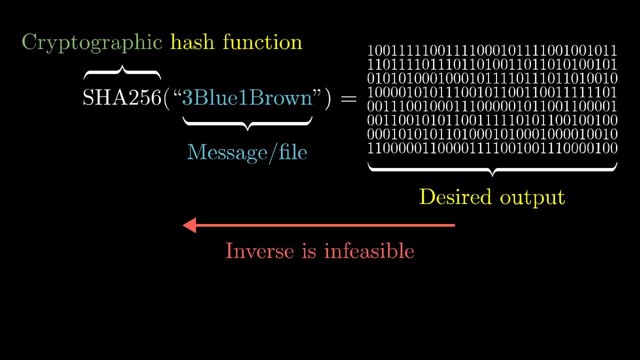 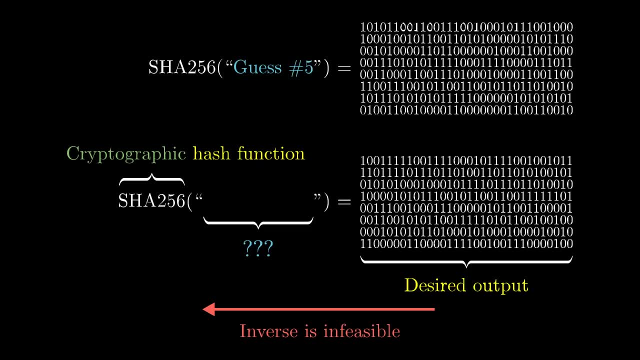 a cryptographic hash function. For example, if you want to find a message whose SHA-256 hash is some specific string of 256 bits, you have no better method than to just guess and check random messages, And this would require on average 2 to the 256 guesses. 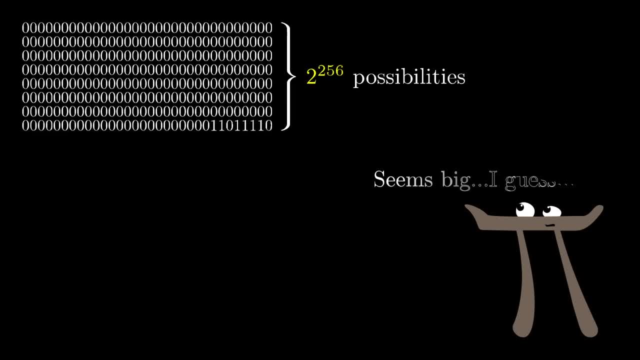 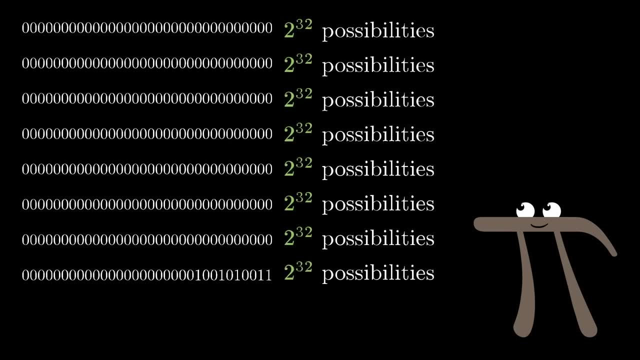 This is a number so far removed from anything we ever deal with that it can be hard to appreciate its size. But let's give it a try. 2 to the 256 is the same as 2 to the 32, multiplied by itself 8 times. 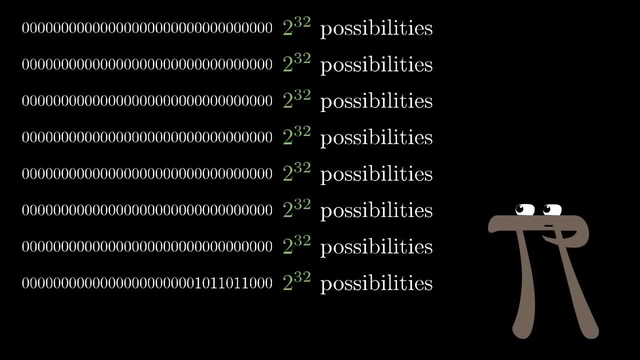 Now what's nice about that split is that 2 to the 32 is the same as 2 to the 32 multiplied by itself. 8 times 2 to the 32 is 4 billion, which is at least a number we can think about. right, It's the. 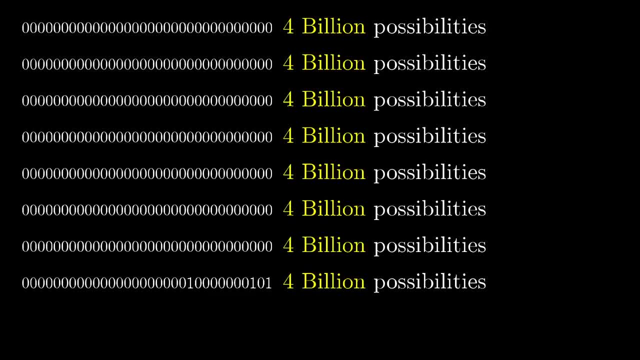 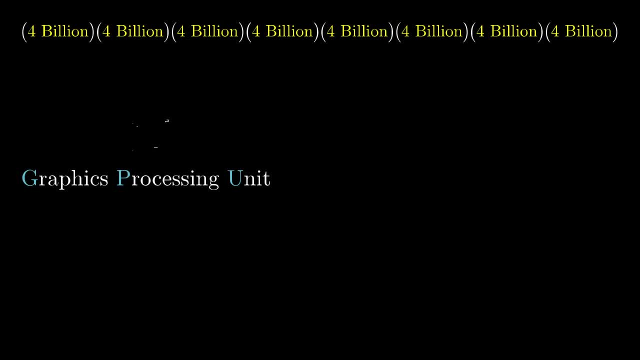 kind of thing you might see in a headline. So all we need to do is appreciate what multiplying 4 billion times, itself 8 successive times, really feels like. As many of you know, the GPU on your computer can let you run a whole bunch of computations. 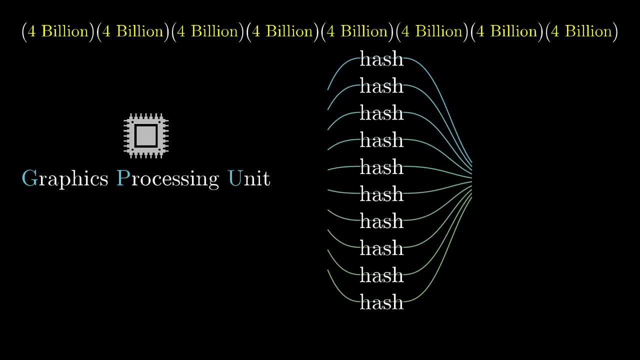 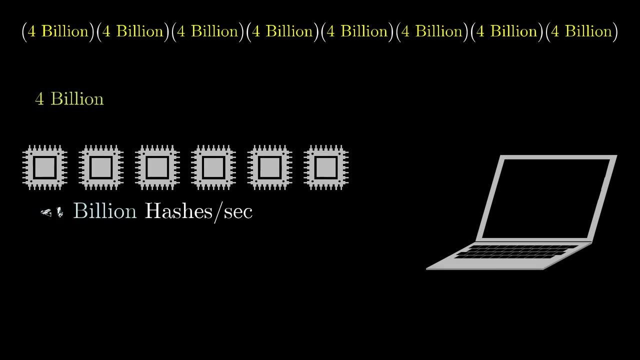 in parallel incredibly quickly. So if you were to specially program a GPU to run a cryptographic hash function over and over a really good one, might be able to do a little less than a billion. And let's say you just cram your laptop around for a bunch of extra GPUs. so your laptop 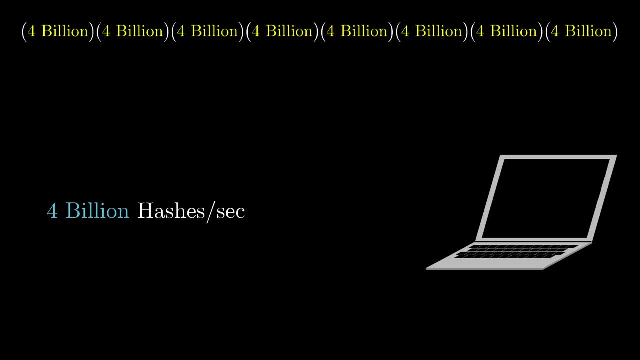 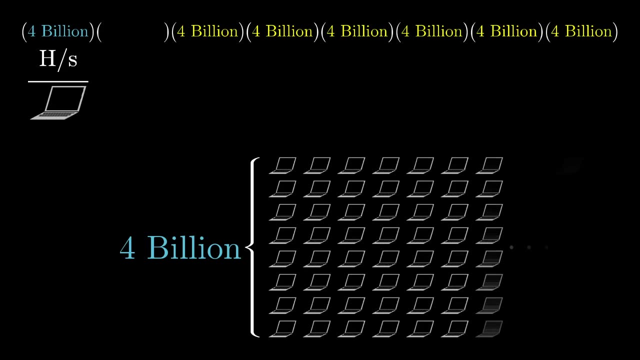 can run 4 billion. So these first 4 billion represent the number of hashes per seconds per computer. Now picture 4 billion of these GPU-packed computers. For comparison, even though Google doesn't make their number of servers public at all, estimates go somewhere in the single-digit millions. 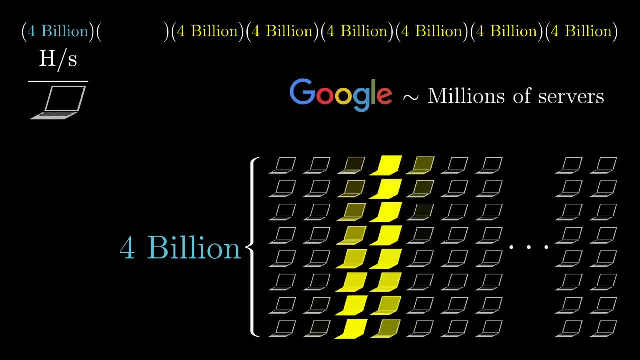 In reality, most of those servers are going to be much less powerful than our imagined GPU-packed machine. but let's say that Google replaced all of its millions of servers with a machine like this, then 4 billion machines would mean about a thousand copies of this. 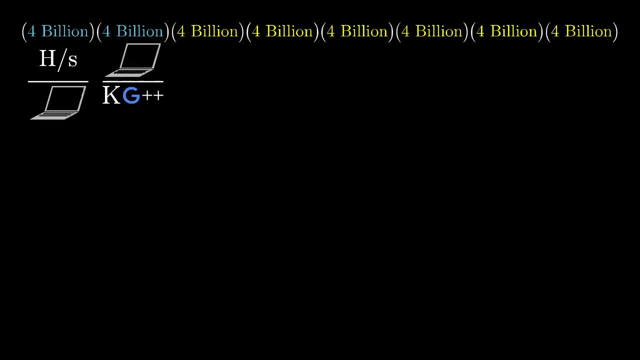 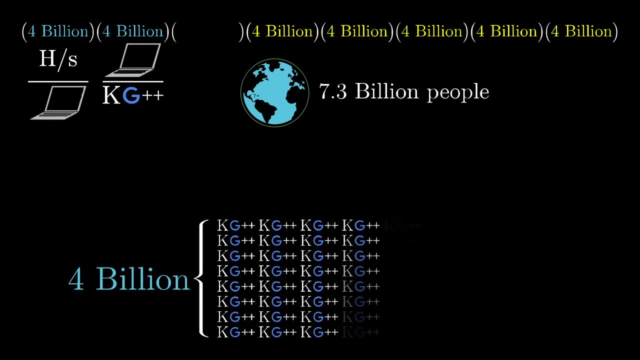 souped up Google. Let's call that one KillaGoogle. worth of computing power, There's about 7.3 billion people on Earth, So next, imagine giving a little over half of every individual on Earth their own personal KillaGoogle. 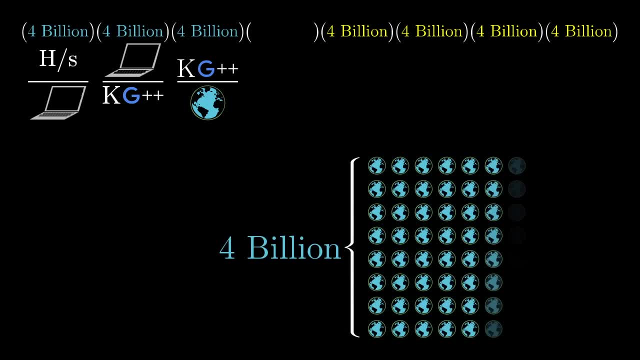 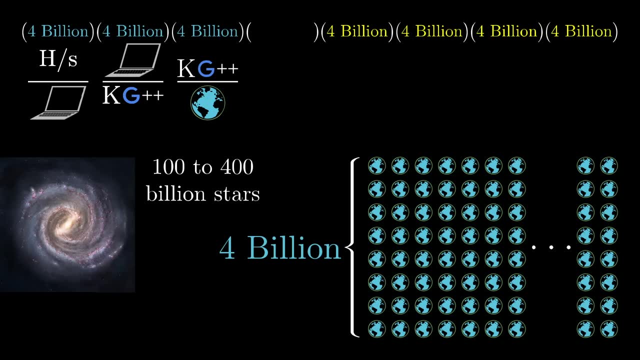 Now imagine 4 billion copies of this Earth. For comparison, the Milky Way has somewhere between 100 and 400 billion stars. We don't really know, but the estimates tend to be in that range. So this would be akin to a full 1% of every star in the galaxy having a copy of Earth. 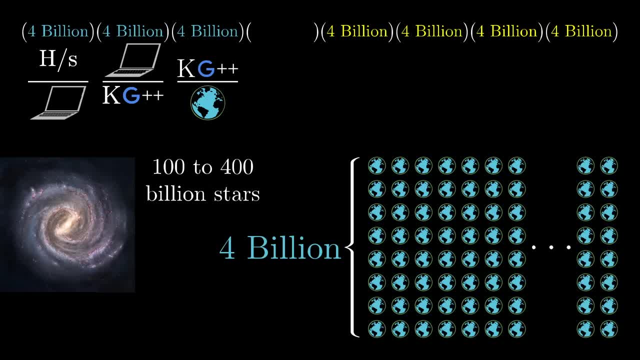 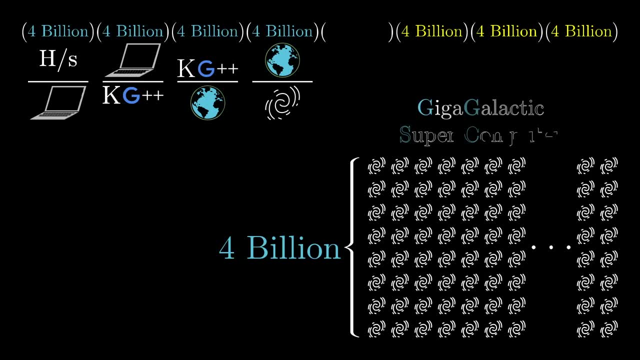 where half the people on that Earth have their own personal KillaGoogle. Next, try to imagine 4 billion copies of the Milky Way, And we're going to call this your gigagalactic supercomputer, running about 2 to the 160. 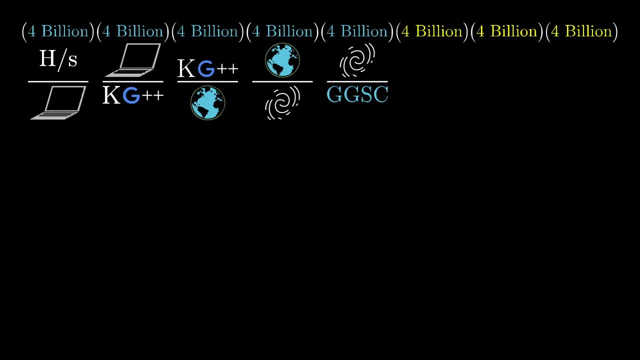 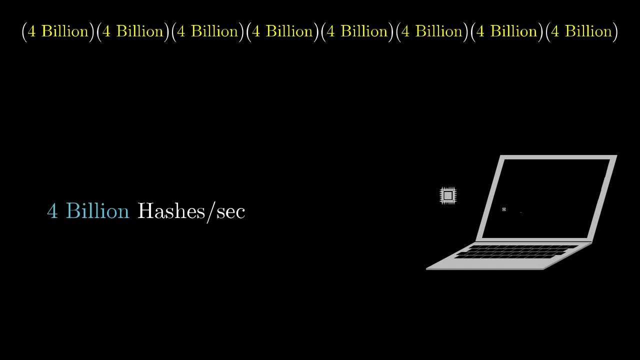 guesses every second. Now, 4 billion seconds, that's about 126.8 years. 4 billion of those, well, that's 507 billion years, which is about 37 times the age of the universe. So even if you were to have your GPU-packed KillaGoogle-per-person multi-planetary gigagalactic. 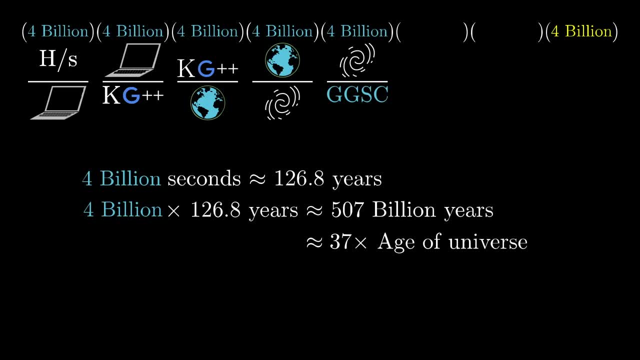 computer guessing numbers for 37 times the age of the universe. that's only going to be 1 in 4 billion. If you had your GPU-packed KillaGoogle-per-person multi-planetary gigagalactic computer guessing numbers, it would still have only 1 in 4 billion of the correct guesses. 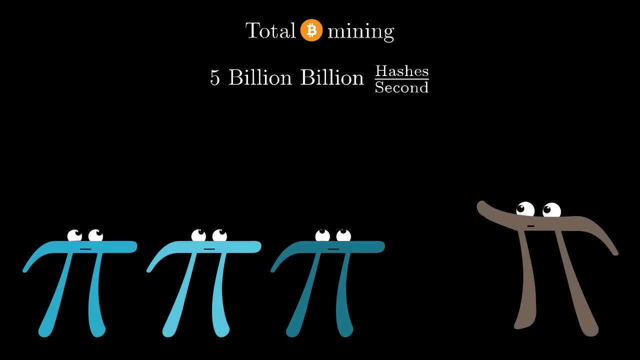 By the way, the state of Bitcoin hashing these days is that all of the miners put together guess and check at a rate of about 5 billion billion hashes per second. That corresponds to 1 third of what I just described as a KillaGoogle. 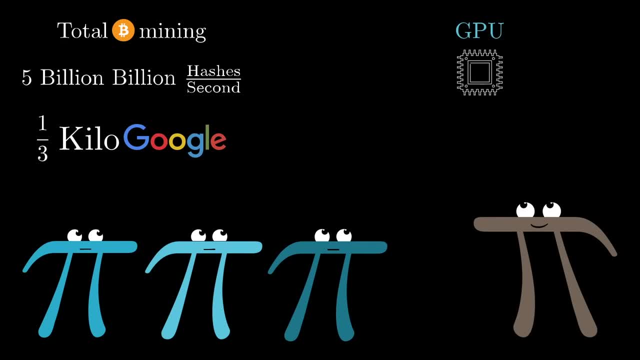 This is not because there are actually billions of GPU-packed machines out there, but because miners actually use something that's not KillaGoogle, something that's about a thousand times better than a GPU Application-specific integrated circuits. These are pieces of hardware specifically designed for Bitcoin mining. 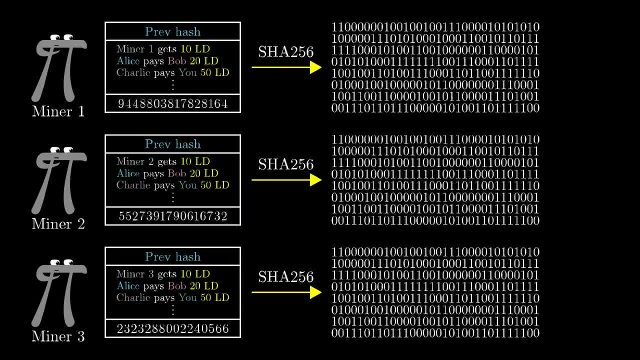 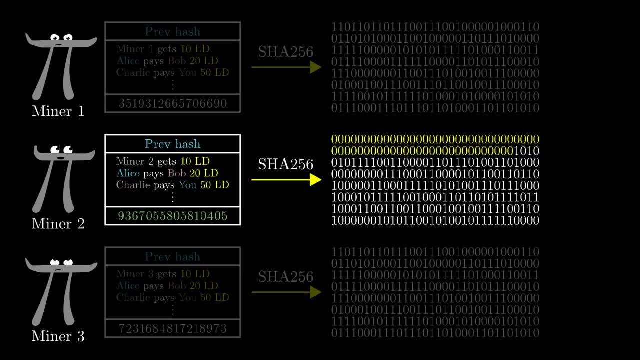 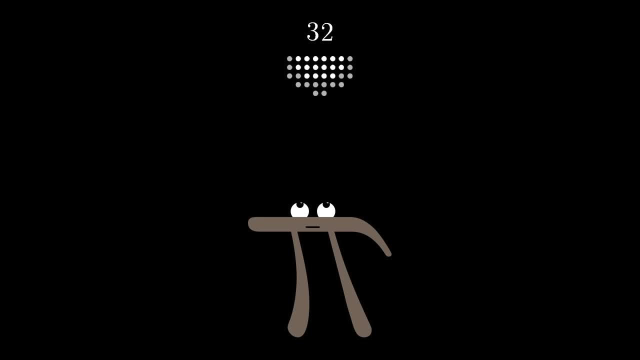 for running a bunch of SHA-256 hashes and nothing else Turns out. there's a lot of efficiency gains to be had when you throw out the need for general computation and design your integrated circuits for one and only one task. Also on the topic of large powers of two that I personally find it hard.